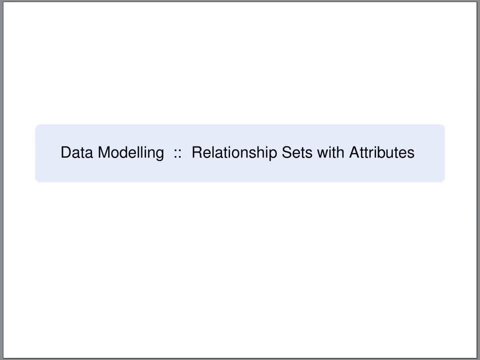 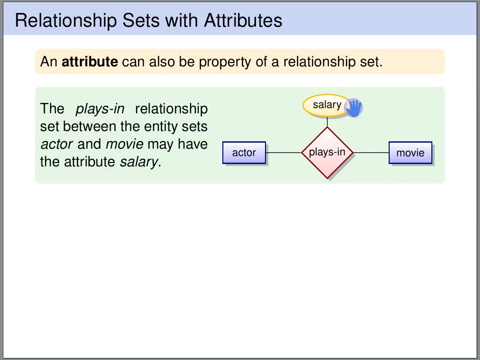 We've already seen that attributes can be connected to entity sets, But also relationship sets can have attributes. For instance, the place in relationship set that we've seen before could be equipped with an attribute salary, So we can express that a certain actor has earned a certain salary for playing in a certain movie. This is the example that 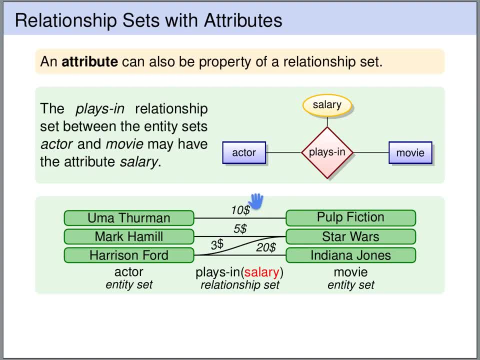 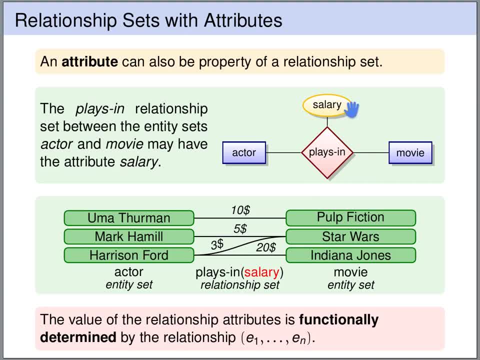 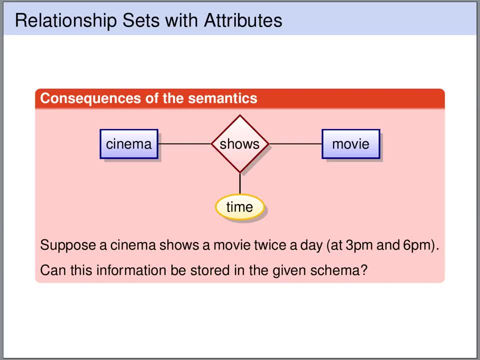 This functionally determines the salary. This functional determination has an important impact on our design. So, for instance, assume that we want to make a database of cinemas and movies and we want to encode information- what cinema shows what movie at what time. So we have entity sets cinema and an entity set movie. 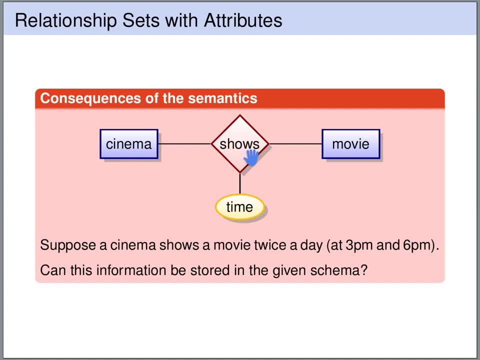 And we have a relationship set shows, And this relationship set shows has an attribute time. Now we of course have cinemas that show certain movies more than once a day, let's say at 3 and at 6 pm, And the question is: can this information be stored in this schema? 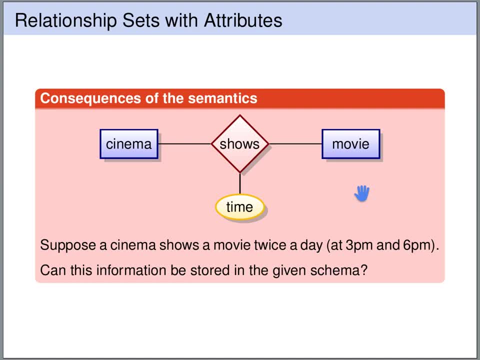 And the answer is no, Because the value of the attribute time is functionally determined by the participating entities. So it's functionally determined by the cinema and the movie. So if I tell you the cinema and the movie, then there's only one time at which the movie can play.